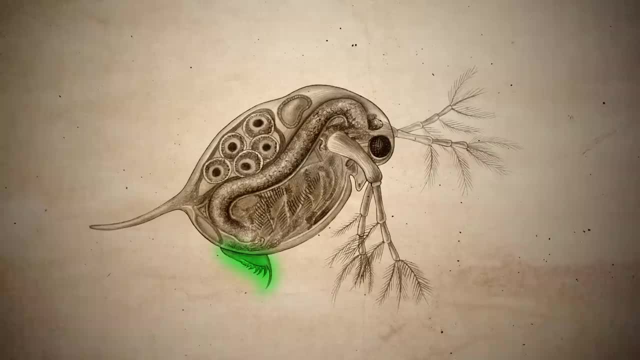 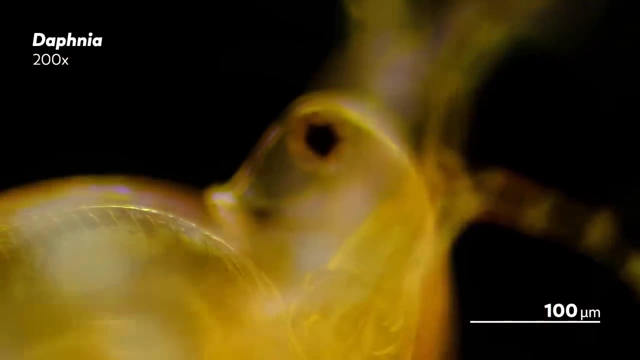 There's also an array of five to six limbs that form a feeding and respiratory apparatus, As well as a pair of claws at the end of their abdomen, which they use as a filtering tool or for defense. What might be especially striking is that one very large eye, Something we don't. 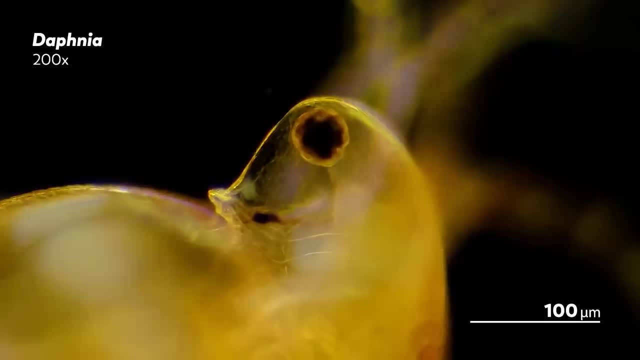 often see in the microcosmos. As embryos, Cladocerans have two brown eye spots, But in the last stage of their development the eye spots merge together to form one large compound eye eye that will go on to help orient them while they swim around. 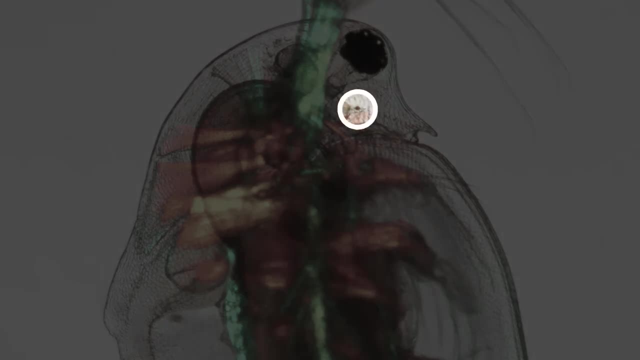 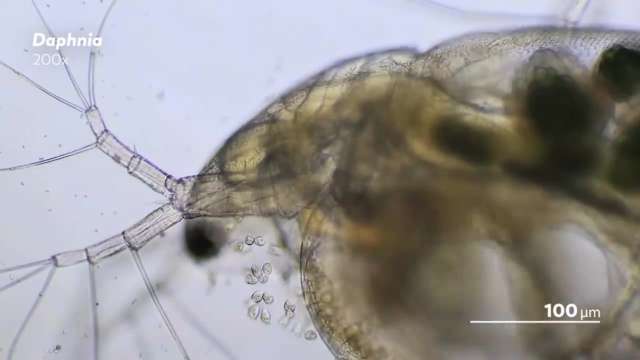 Cladocerans also have another small photosensitive organ called the noplar eye, which is located between the compound eye and the mouth. The water fleas we see most in our journey through the microcosmos are Daphnia, a genus. 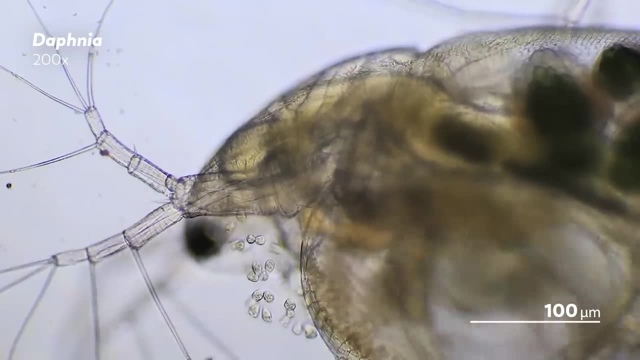 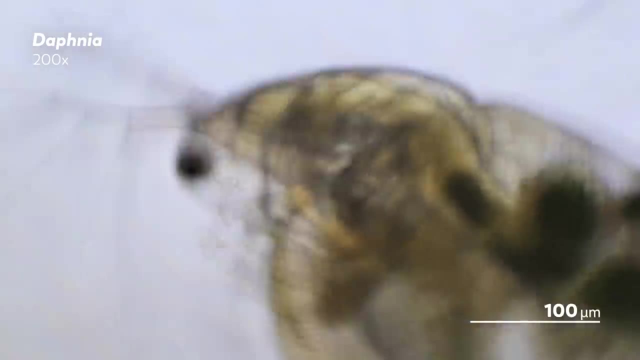 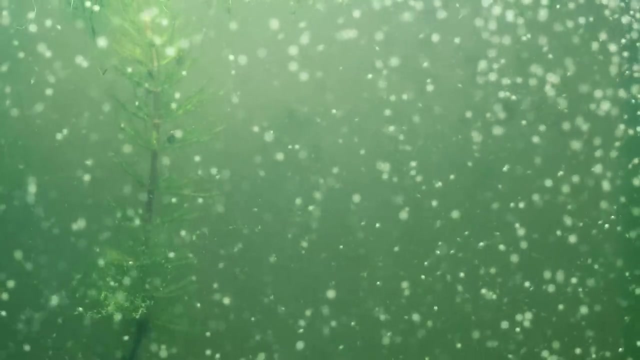 that includes more than 100 species. And while, yes, Daphnia are found in lakes, they're also sold in aquarium stores because fish love to eat them. You might see bags of them filled with hundreds of Daphnia. As they get packed together, the oxygen around them gets depleted. Cladocerans use hemoglobin to transport oxygen and in situations like this they can increase the concentration of hemoglobin in their bodies up to 20-fold to transport more oxygen And as that happens, you might actually see those packs of daphnia become a much more. 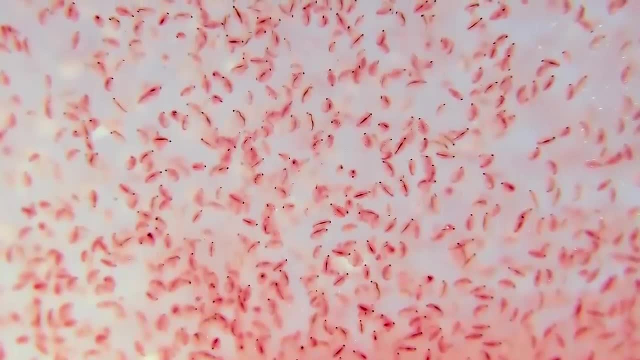 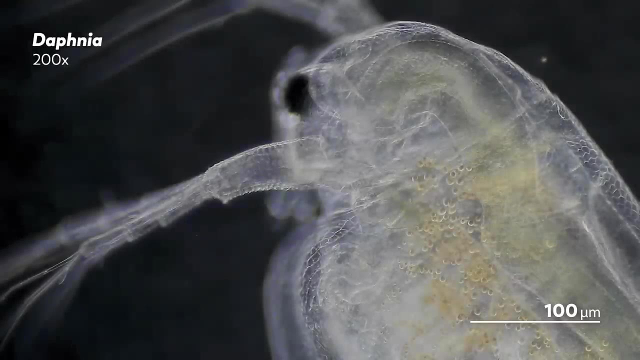 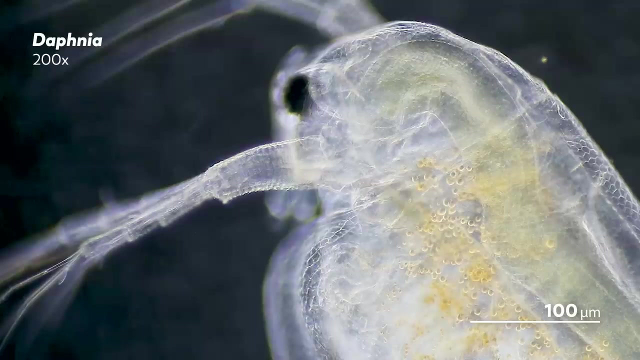 vivid red. Here you can see the daphnia's heart beating. At 20 degrees Celsius it'll beat around 200 times a minute, But that rate depends on the temperature. It beats slower when the daphnia are in colder conditions. 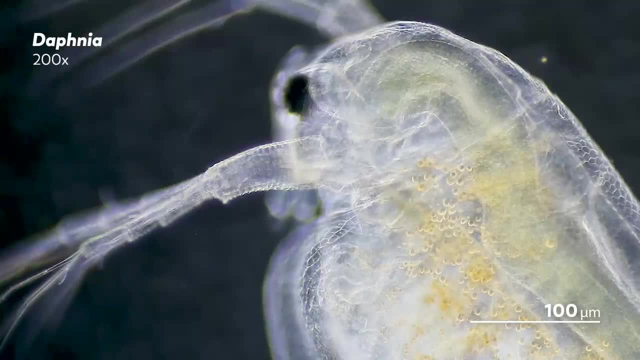 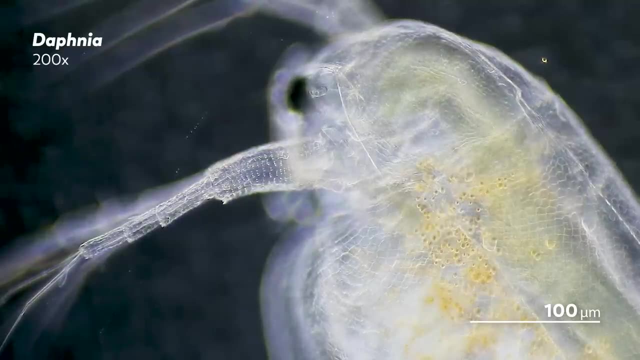 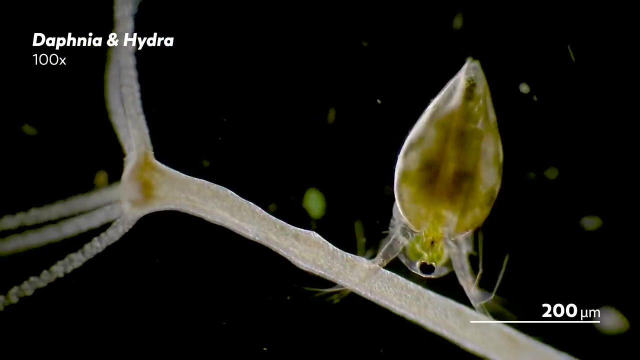 The heart rate will also change in the presence of substances like alcohol and caffeine. But we were a little bit too nervous about hurting our daphnia to demonstrate that Our daphnia often come from those aquarium packs rescued from their fate as fish food. 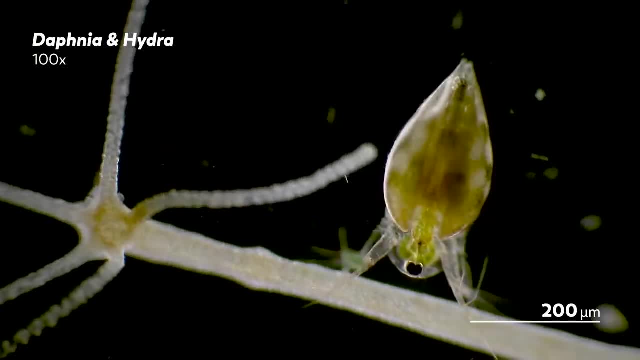 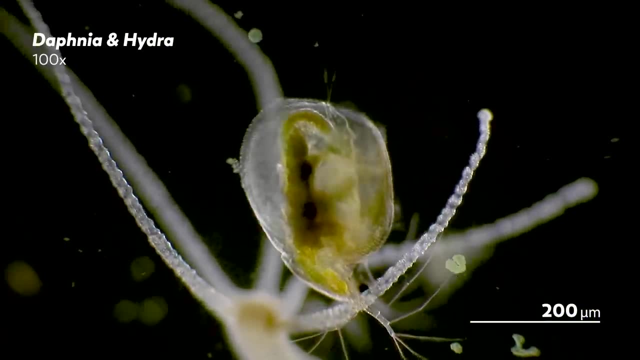 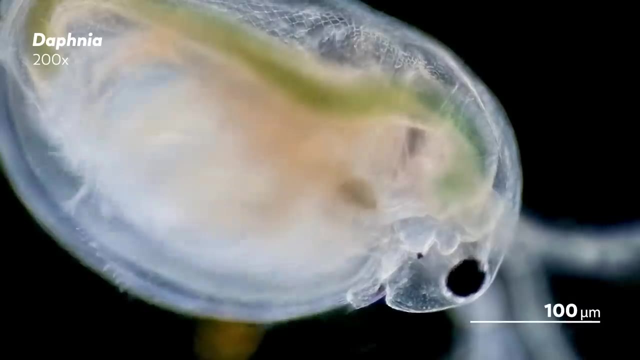 to live a less hazardous life in our own fish-free pond aquarium. They do occasionally get eaten by the hydra, But it's a better chance of survival compared with the alternative. Daphnia and their cladocerin relatives are filter feeders gathering their food with. 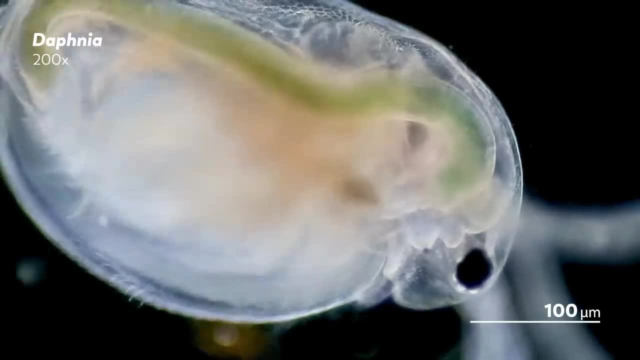 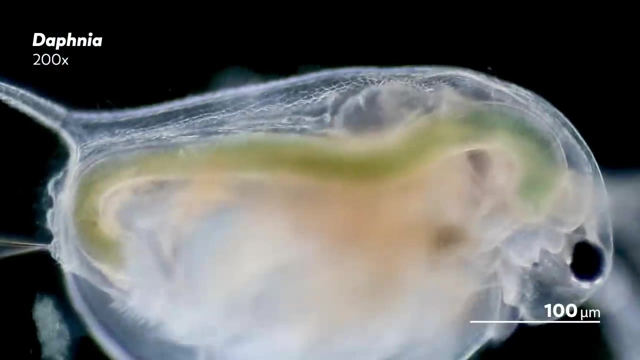 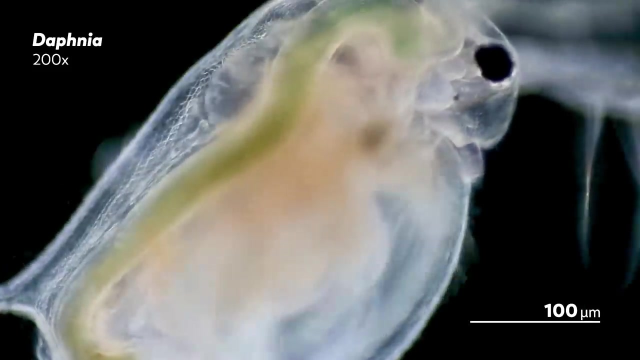 a filtering apparatus made of their limbs. Key among these are their phyllopods, a set of flat legs that resemble leaves. The phyllopods create a water current that flows from the front of the water flea towards the back, allowing it to collect and consume algae. 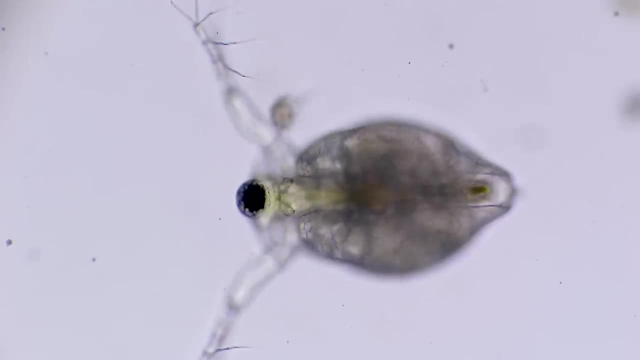 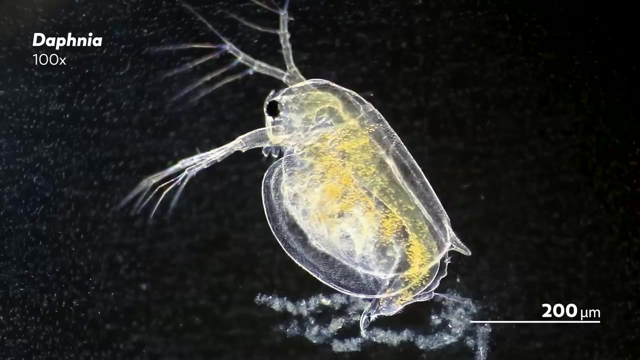 Here you can see a daphnia filtering a rotifer, Though the rotifer is quickly discarded, probably because it's a bit too big for easy consumption. While daphnia are often transparent, you can sometimes get hints of just what food is dominating. 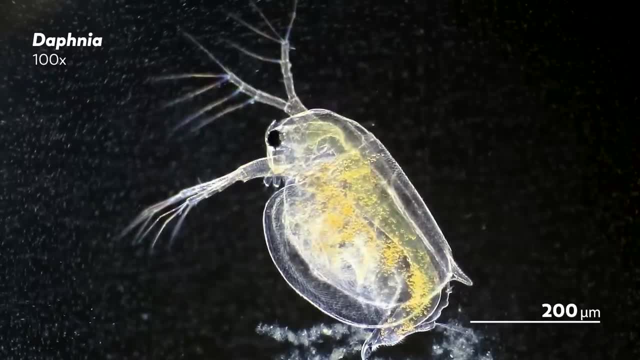 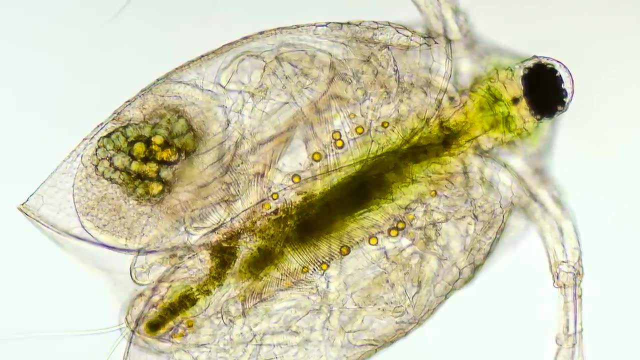 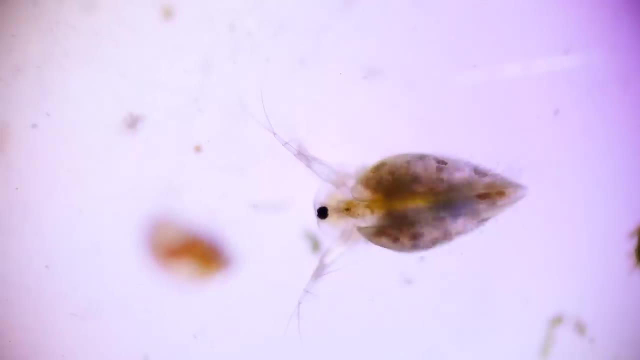 their diet by looking at the tinges of color that line their body. With more green algae, the daphnia will start to look a little green or yellow. When they eat more bacteria you might see more of a white or salmon pink color. 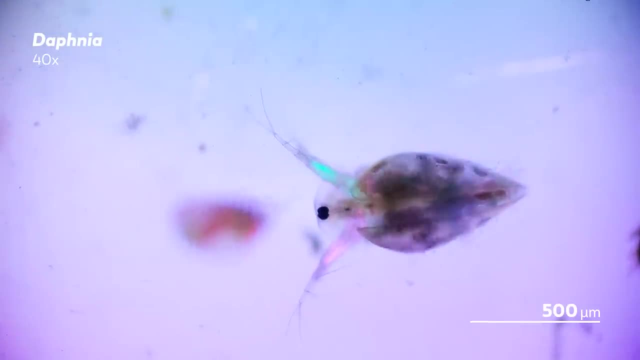 Daphnia are, of course, often eaten, so they employ several strategies to avoid predators, including the tried and true strategy of just getting the heck out of the way. Only when daphnia do it, we call it dial vertical migration. 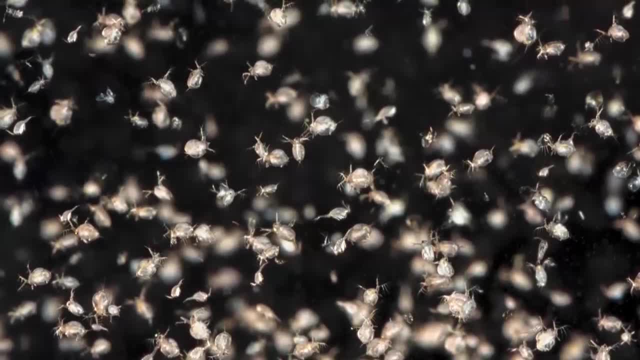 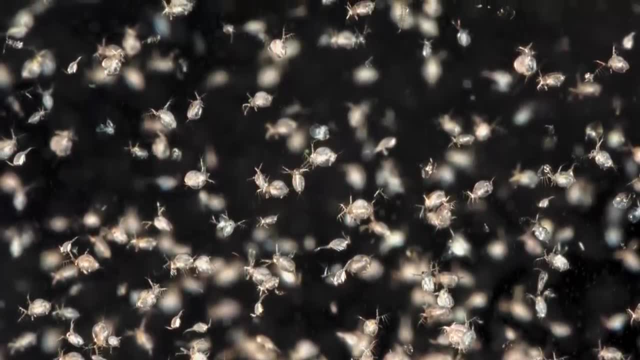 During the day, when light is peaking, they're more likely to eat the daphnia that are in the water. White is plentiful. They stake out lower, darker depths where predators are less able to see them. During the night, they move upwards, able to eat without fear of looming threats. 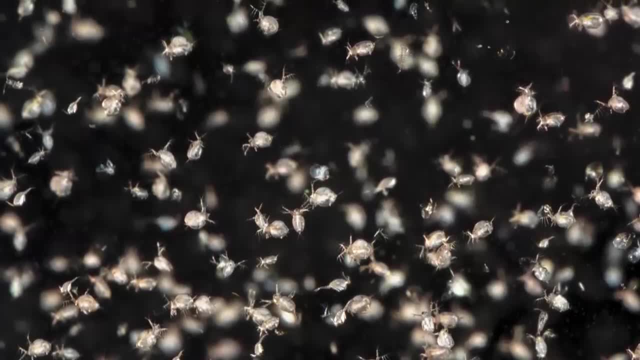 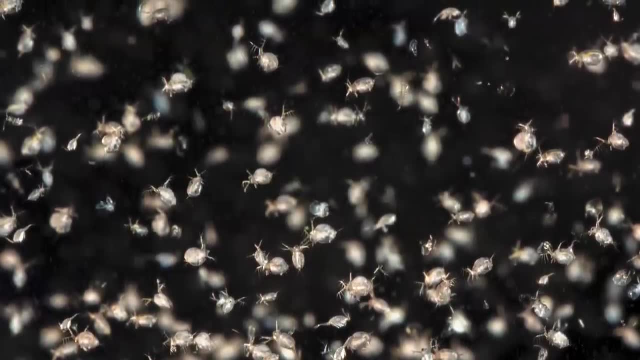 Daphnia arrange this dial-vertical migration around the presence of fish chiromones. Chiromones are chemical signals that alert them to the proximity of fish. If they don't detect these signals, the daphnia might just spend the day hanging out. 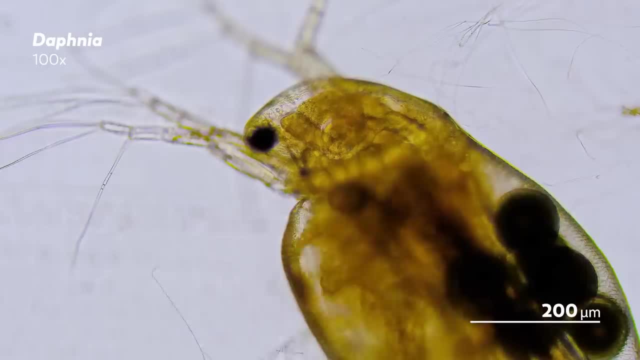 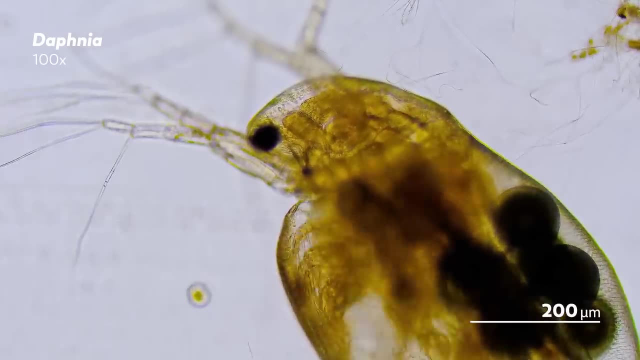 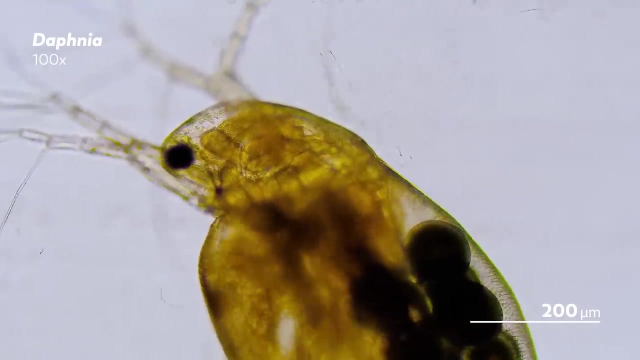 towards the surface so they can gather more food. But chiromones don't just affect the daphnia's migration, They also affect the size of their offspring. In the presence of fish, chiromones- one daphnia species- has been observed birthing smaller. 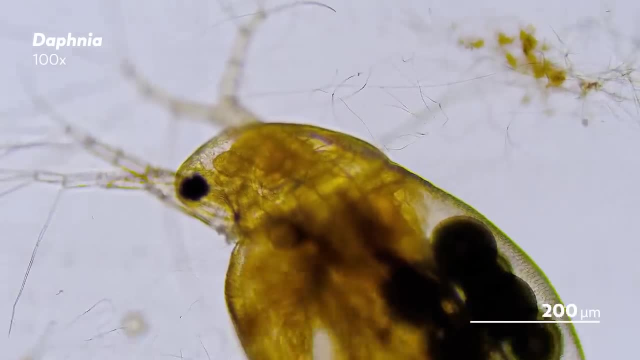 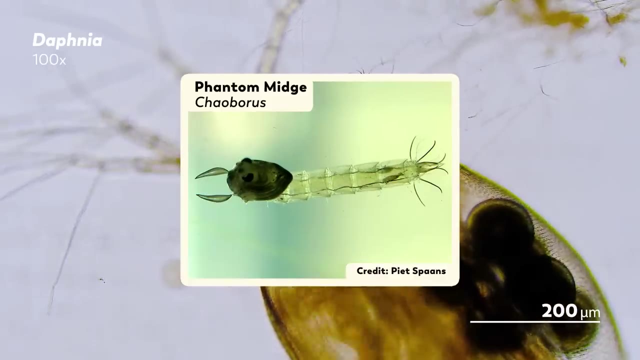 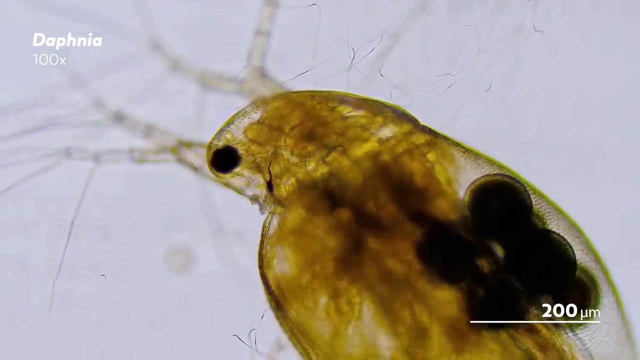 water fleas, a change in size that helps them avoid detection. Interestingly, though, the presence of the phantom midge, another predator, sets off the opposite. As a result, their chiromones will make the daphnia grow larger, presumably because the 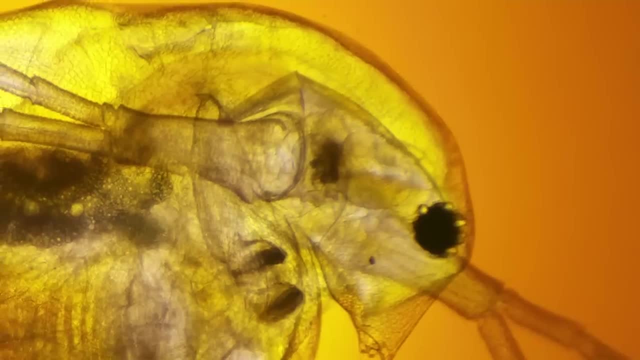 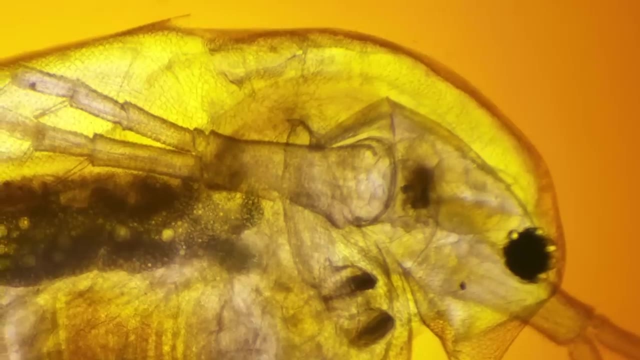 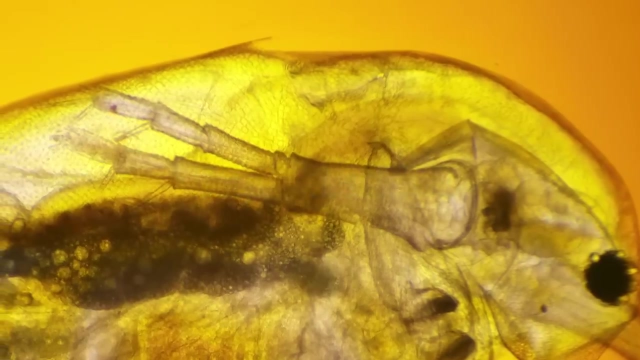 midge prefers a smaller prey. In response to the midge's chiromones, the daphnia have also been observed growing a set of jagged edges on their head called neck teeth. You know all the usual protective measures: Growing extra large and having teeth on your neck. 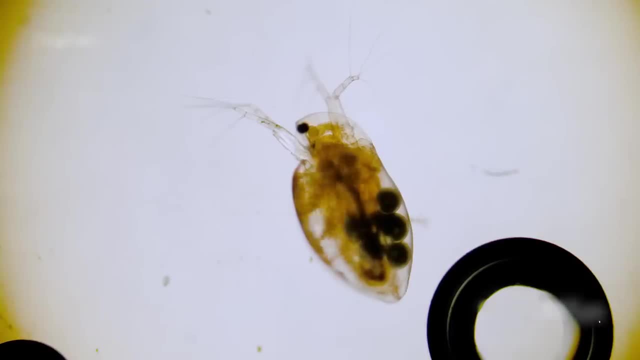 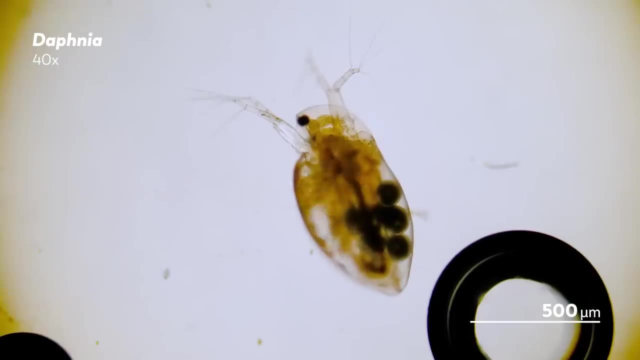 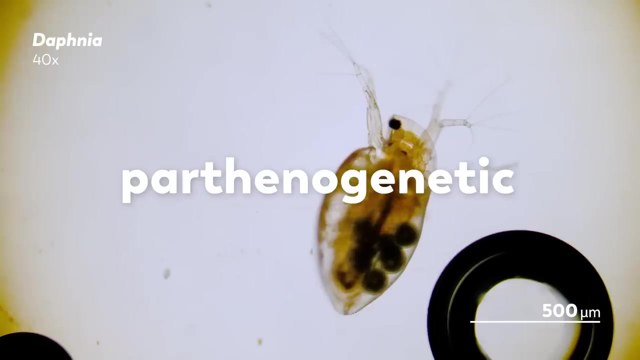 Environmental cues. These cues also shape the reproduction of daphnia by directly affecting the sexual composition of their population. An adult female daphnia will usually go through asexual reproduction, producing a clutch of parthogenetic eggs every time she molts. The eggs go into her brood chamber and after about a day they hatch. The young larvae stay inside her brood chamber for about three more days, emerging as young daphnia. They're not born until the end of the egg. That's the first of their population, the oldest of the two. 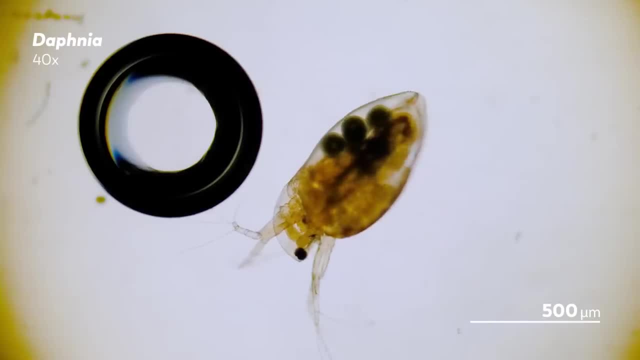 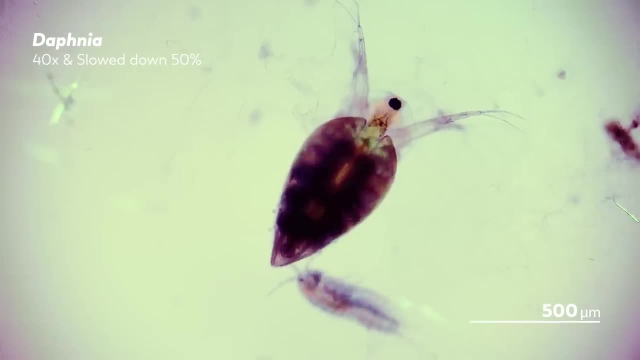 With asexual reproduction. a female daphnia might produce a clutch every three to four days until her death, producing more clones of herself and rapidly increasing their population. There are a few daphnia species that are strictly parthenogenetic, but most follow a pattern. 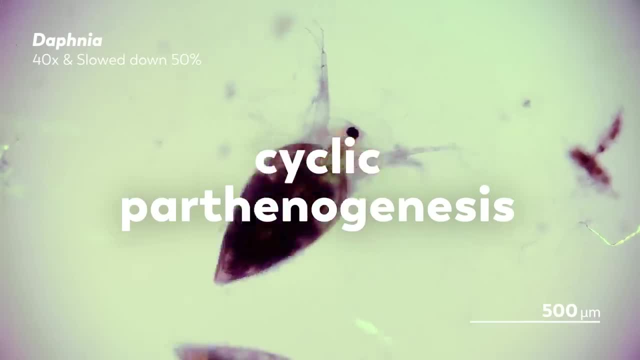 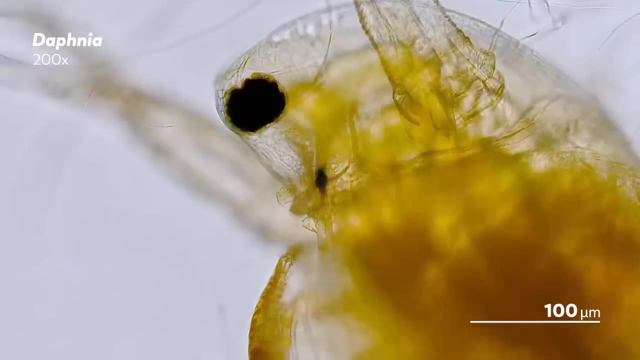 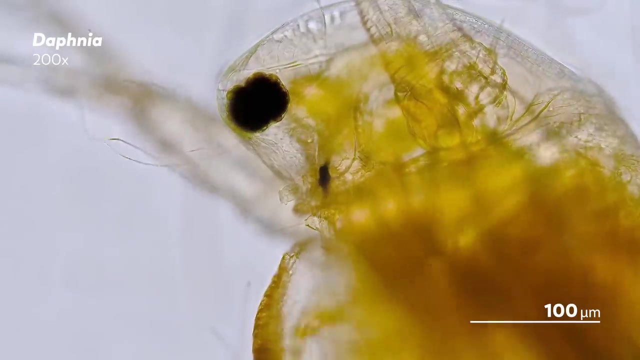 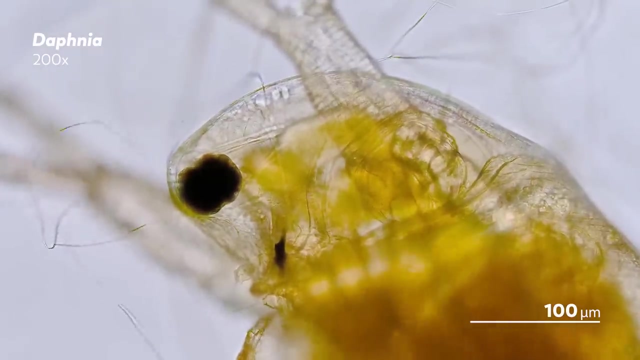 called cyclic parthenogenesis, interrupting their asexual cycle for sexual reproduction, which happens in response to environmental cues, signaling that times have gotten tough. Maybe the population has become too dense and their food has become scarce, Or perhaps the days are getting shorter, the temperature is lower or the pond drier. 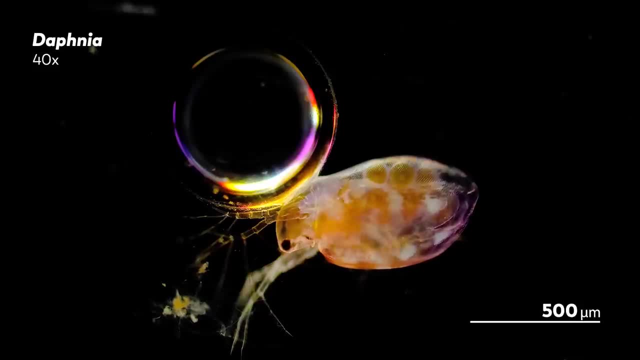 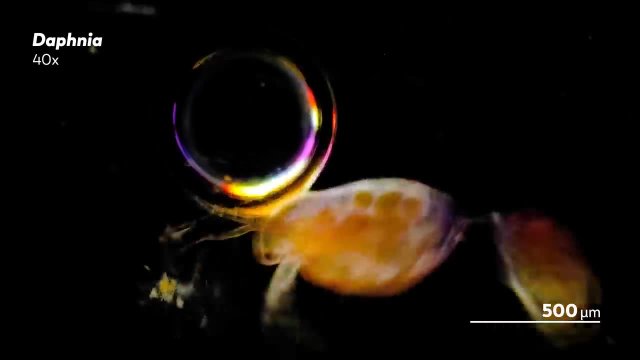 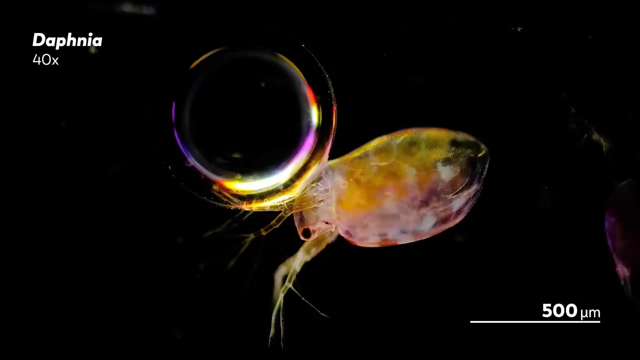 When these external danger signals are sensed, some of the parthogenetically-derived eggs will start to hatch into males. These male Daphnia are genetically identical to their female broodmates. After all, they are parthenogenetically produced, And that means that sex in Daphnia is an environmentally determined trait. 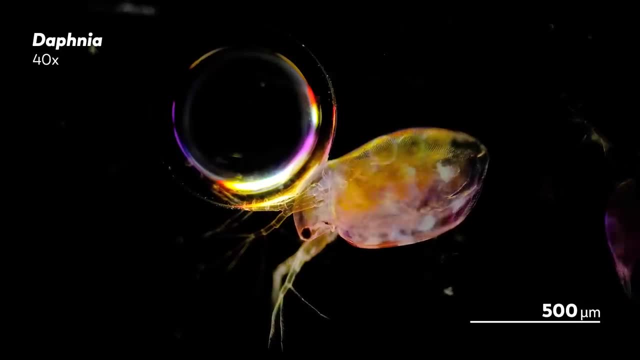 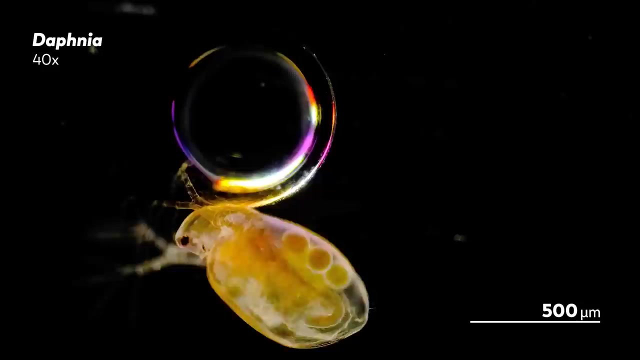 There isn't a genetic difference between males and females. Rather, there's some kind of external signal that takes a genetically identical population of Daphnia and determines whether some of them will become male. Those males then reproduce With females from other clutches, creating an opportunity for true gene exchange. 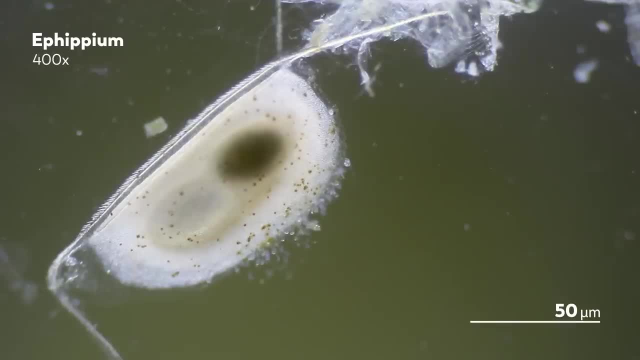 Following sexual reproduction, the female Daphnia will produce a protective saddle-like structure called an aphipium, which holds two eggs called the resting eggs. When the female molts, she will shed the aphipium too. It might sink to the bottom of the pond or disperse through the water or with the wind. 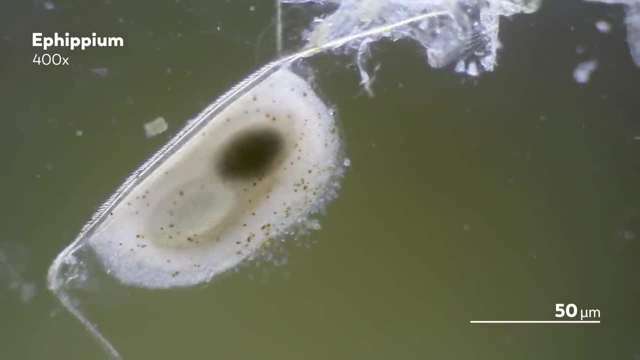 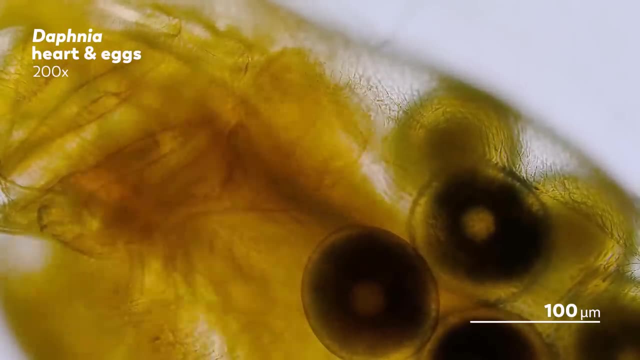 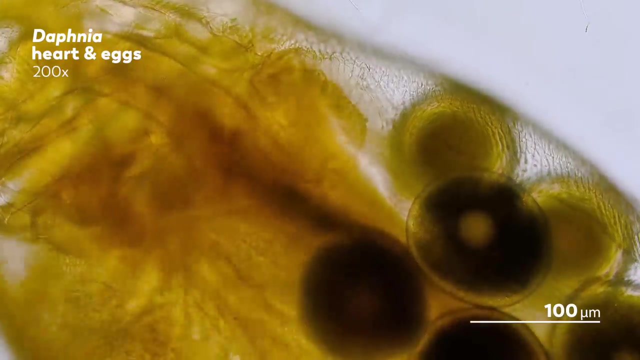 And where it lands, it might rest For years. It's only when the environment that surrounds the egg signals favorable conditions that they will hatch, producing females that will soon proceed back to their normal parthenogenetic reproduction schedule. Nature is full of change. 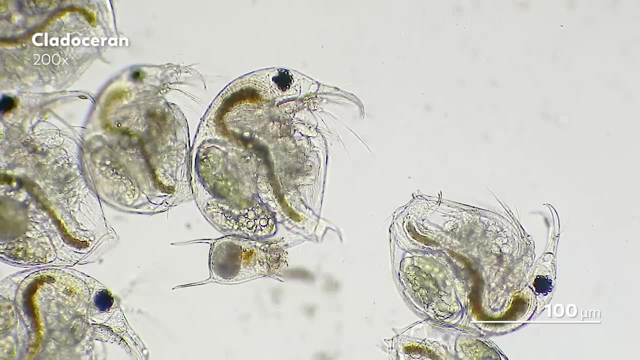 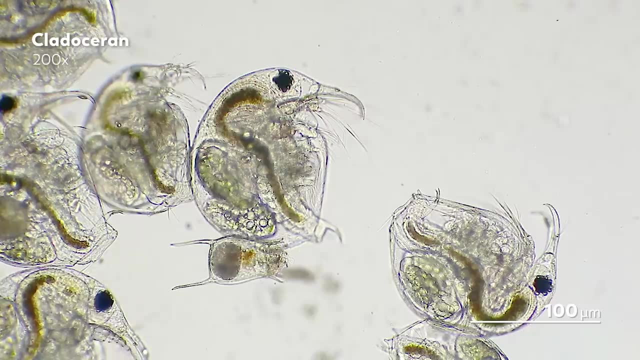 Light temperature, your neighbors. These can alter dramatically over the course of days, weeks and years, And so it's not just about the environment. It's about the environment. The life of any organism, from the smallest microbe to the largest whale, is built on. 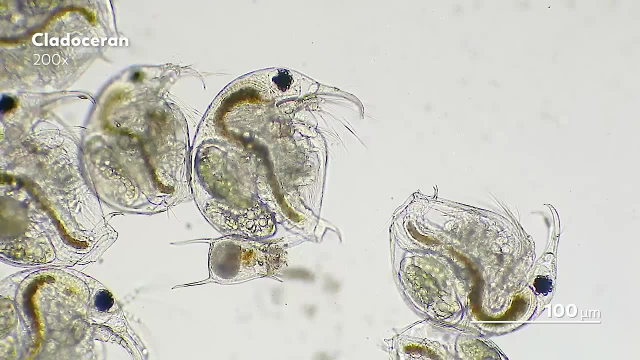 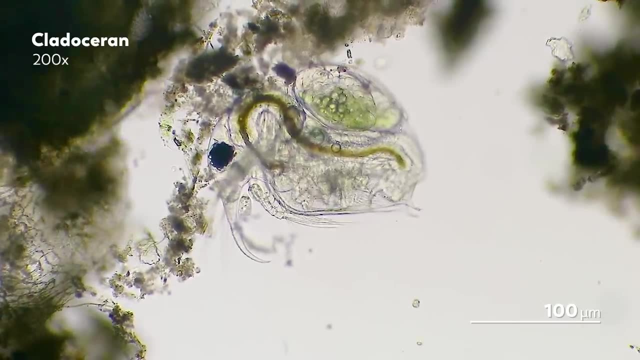 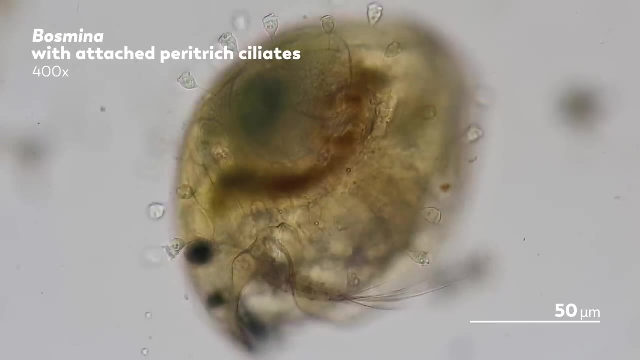 responding and adapting to the changes around them. Compared to many of their smaller neighbors, water fleas don't look like they would be the most nimble in the face of existential threat. In our own footage, they often stand out like awkward giants straddling the thin line. 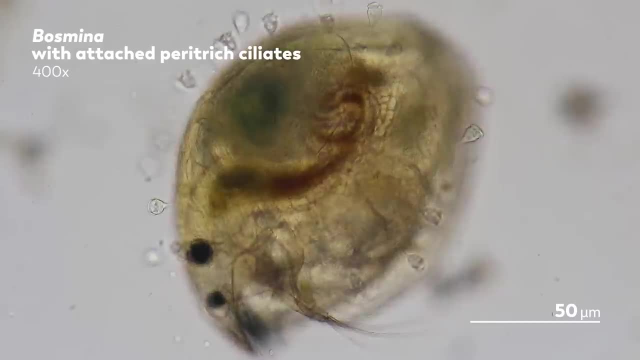 that separates the world of the micro and macro. How could an organism that doesn't quite seem to fit in either world contend with the challenges of both? Quite well, apparently. It's as if they have managed to make the best of both worlds, mastering the reproductive. 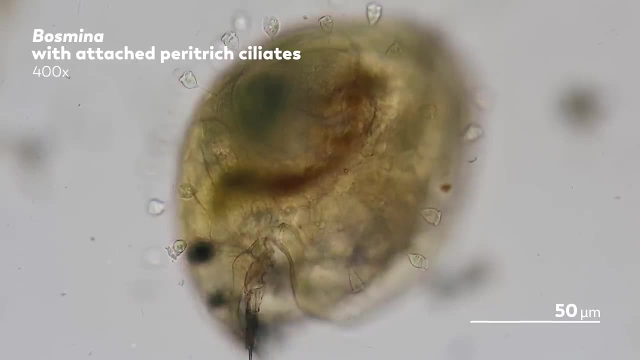 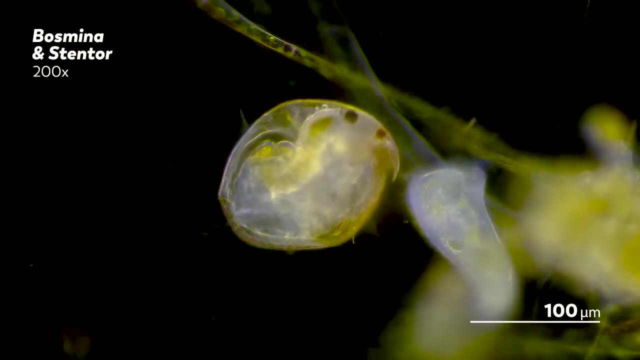 strategies of one while processing the signals of the other. Yes, it is true, water fleas may not be the most elegant of the creatures we see in the microcosmos, But with a bag full of indelible creatures they are. 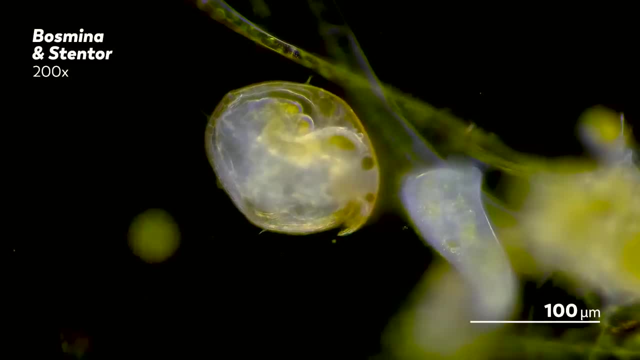 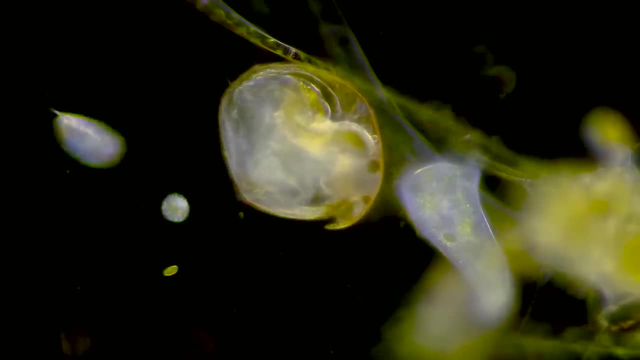 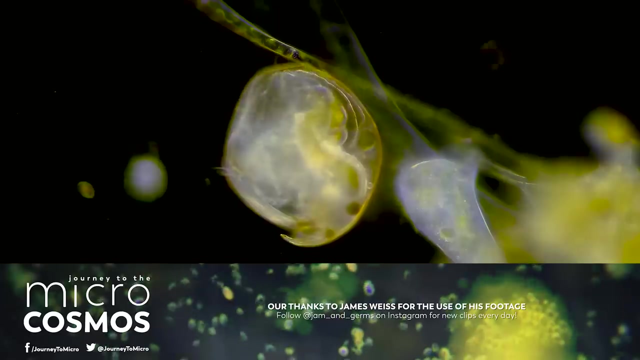 But with a bag full of indelible creatures. they are, And with ingenious tricks, you can't deny that they've got style. Thanks for coming on this journey with us as we explore the unseen world that surrounds us. If you liked this well, that makes us really happy. 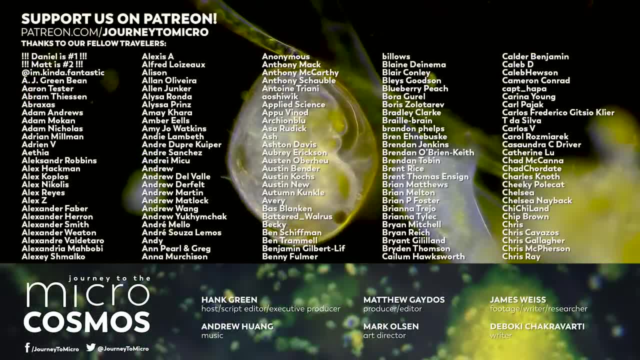 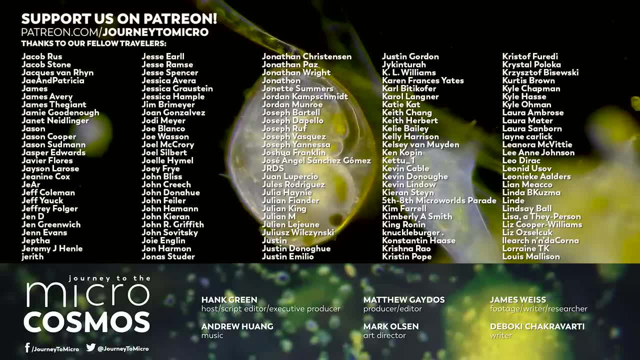 And if you want to thank somebody, you can thank us, But you can also thank all of the people on this screen right now. They are our patrons on Patreon. They are the reason we are able to make this film fun show in these uncertain times of constant change. 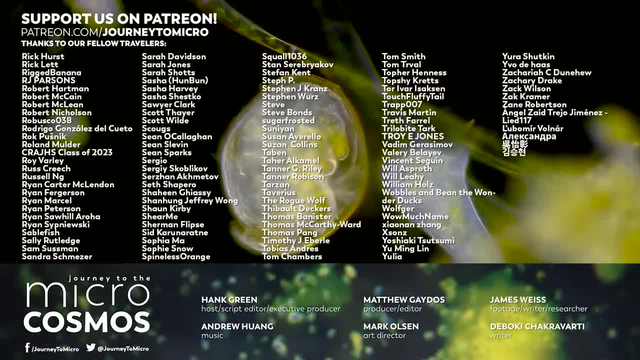 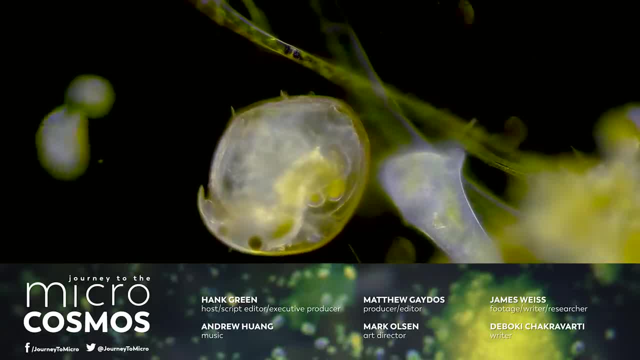 If you want to see more from our Master of Microscopes, James, check out Jam and Germs on Instagram, And if you want to see more from us, we are at youtubecom slash microcosmos. 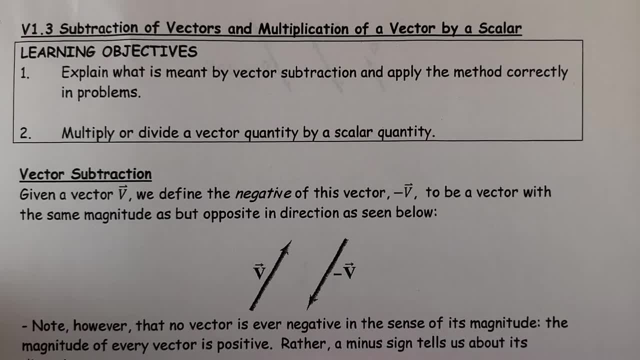 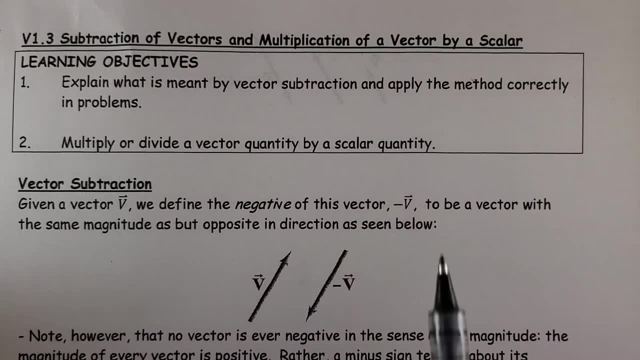 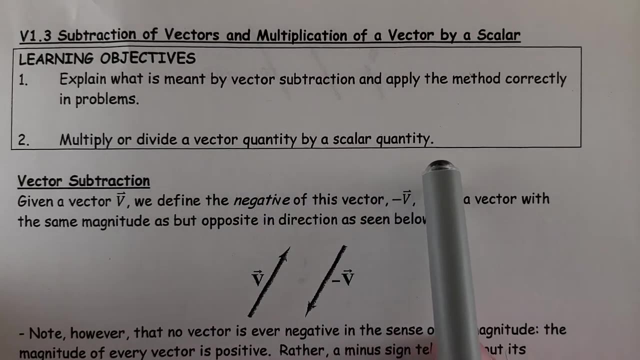 Welcome back to Physics30.. So now we'll look at V1.3: subtraction of vectors: multiplying vectors, dividing by vectors all those operations by a scalar number. So explain what is meant by vector subtraction and apply the method correctly in problems and multiply or divide vectors, quantities, by scalar quantities. 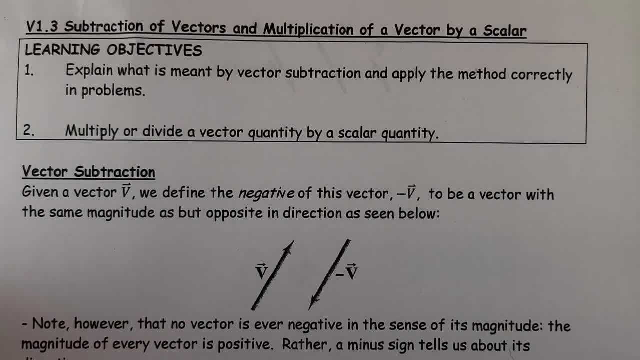 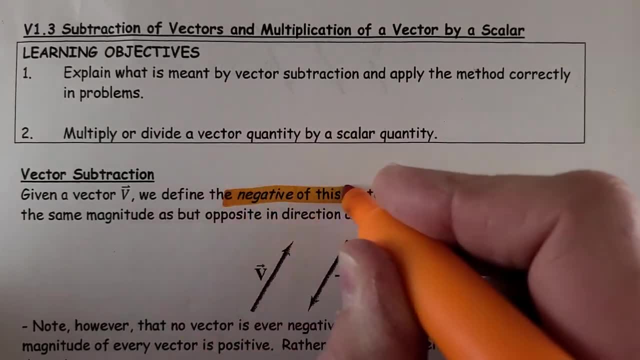 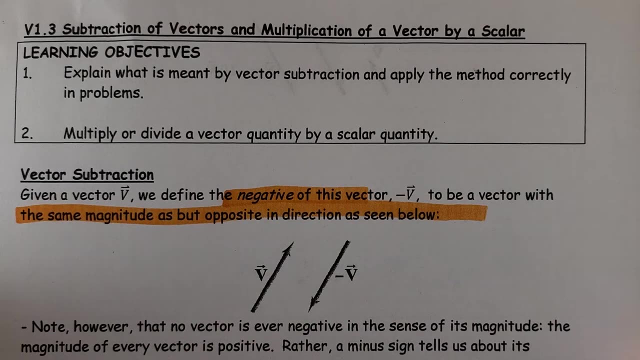 So vector subtraction first of all, given a vector V, we define the negative of that vector to be a vector that has. So the negative of a vector is it has the same magnitude but opposite direction. So this is some vector we can say I don't know, it represents maybe five meters east. 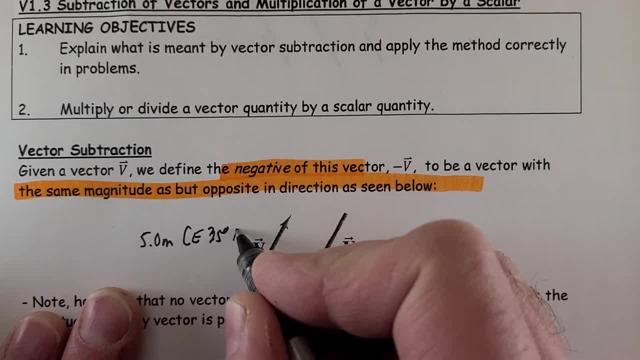 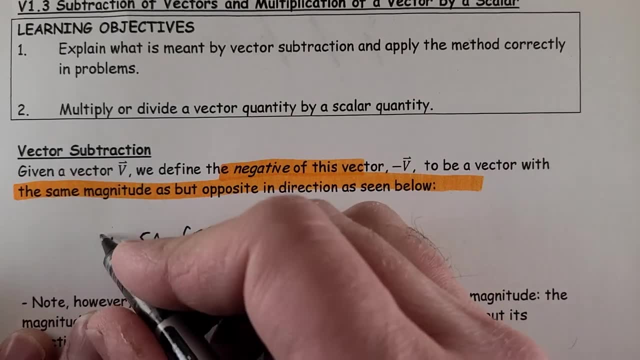 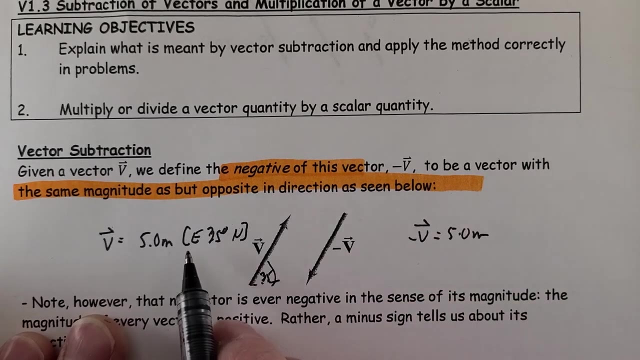 I don't know. looks like maybe 35 degrees north. So if that was 35 degrees north, then the negative of that vector would be it'd still be five, Five point zero meters. So same length, but opposite direction. So instead of east it would be west.